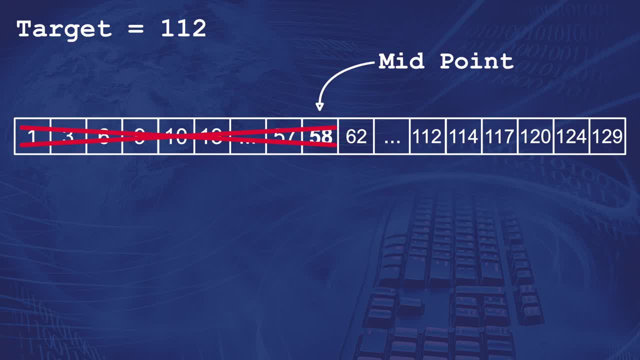 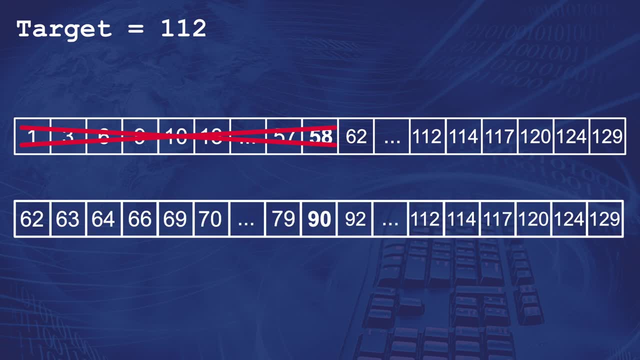 We'll eliminate the entire left half of the list in one guess, And we do this by moving the starting index up to the midpoint. Now we just have half the list, So our next check is to find the new midpoint, which is now number 90.. 90 is lower than 112, so we'll eliminate the left side of the list. 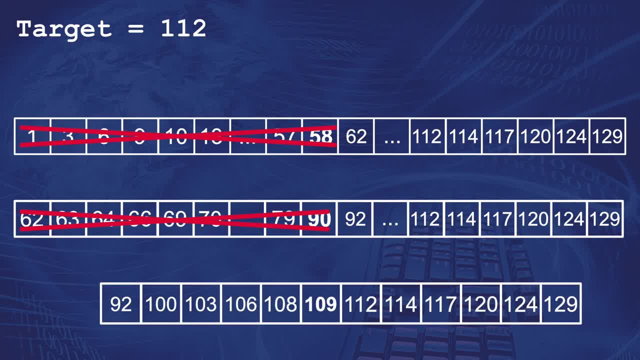 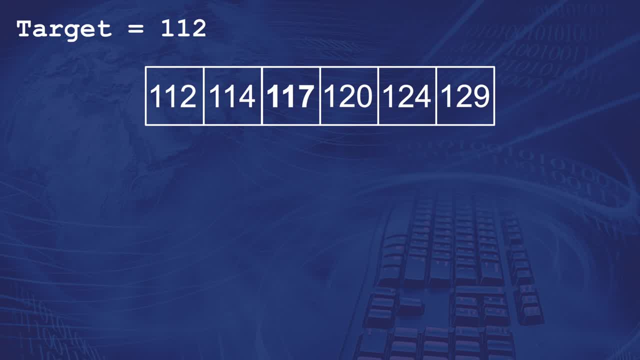 again by moving the starting index up to the midpoint. Next midpoint is 109,, which is lower than 112, wiping out the left side again. And the next midpoint is 117,, which is higher than 112, wiping out the index. So we'll eliminate the left side of the list again by moving the starting. 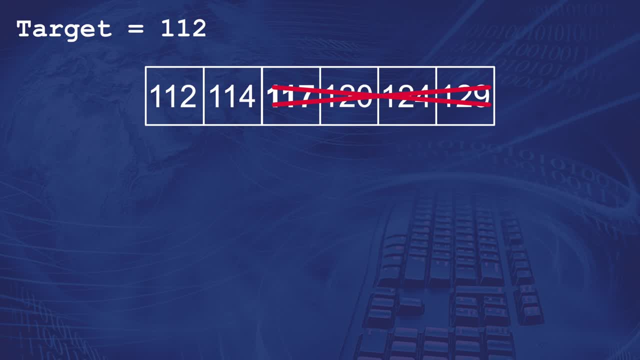 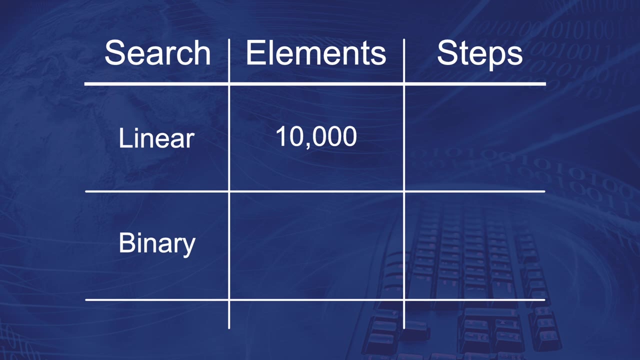 index up to the midpoint And finally we land on index 44, which is 112.. Bingo, we found our number And it only took 5 steps, as opposed to a traditional linear search that would have taken 45 steps. For a little context, a 10,000 element array will take. 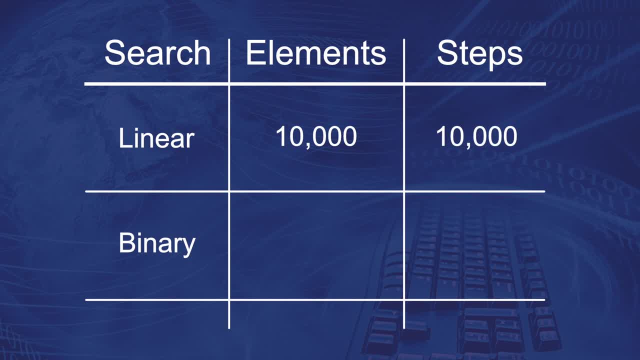 worst case scenario: 10,000 steps for a linear search to find the target, while only 14 steps for a binary search. And as you continue to go up, the binary search gets more efficient, at only 32 steps to find an item in a billion element array. If you want to know why? 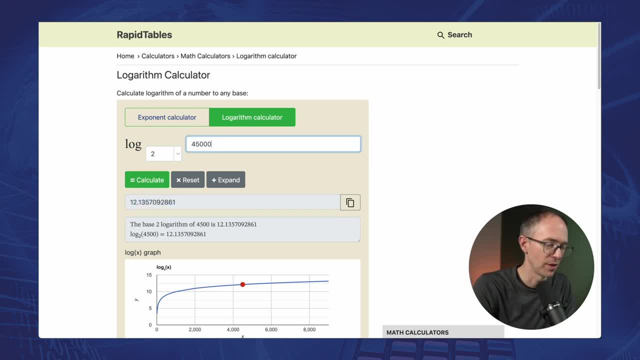 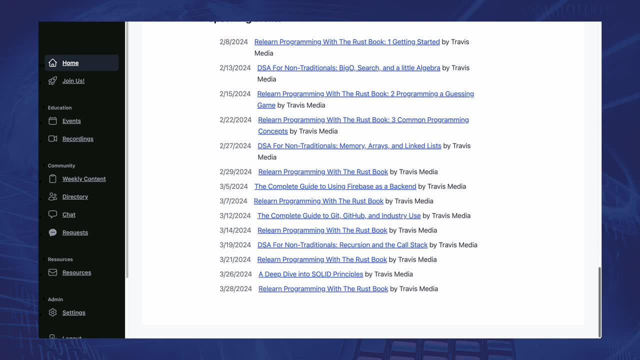 it gets more efficient, or how you can calculate the steps in any binary search and how this all fits into what we call Big O Notation. then check out my weekly Data Structures and Algorithm Events in the Impostor Devs community Link below. And finally, while some languages like C-sharp 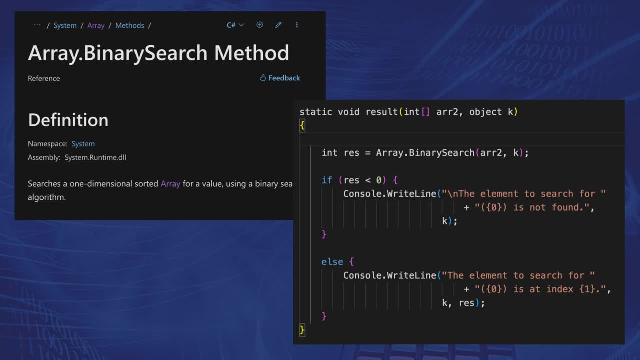 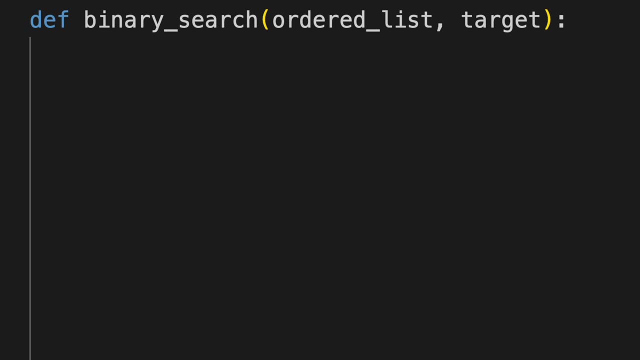 has a binary search built in others. we have to implement them ourselves. So how do we write this in Python? Well, first we define the function. It takes an ordered list and the number we're looking for as parameters. Next we get the size of the list, then the first element of the array. 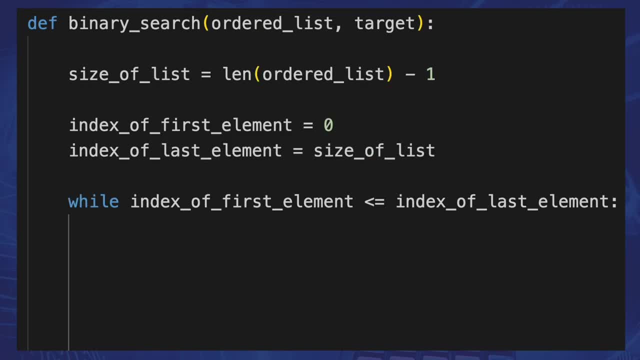 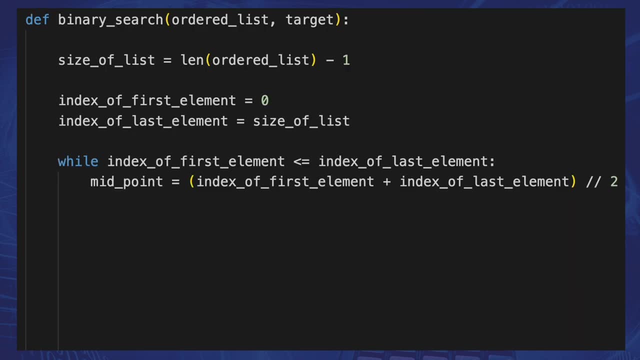 and the last element of the array, And then we create a while loop that continues until the list is small enough, And in this while loop we'll get the midpoint by dividing the sum of the first and the last index by 2.. And to keep it a whole number, we'll do some floor division, hence the 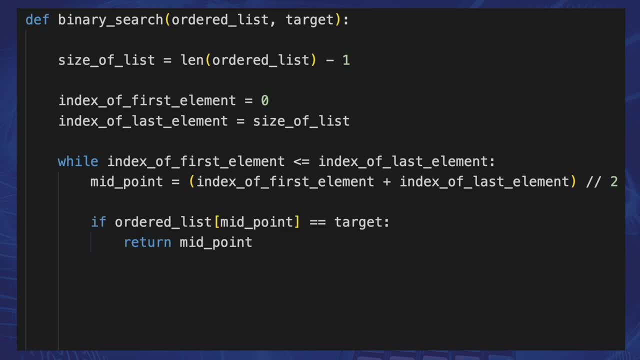 two slashes, Then if that midpoint value equals the target, then we've found the number and we return the number, And that's it. Thanks for watching and I'll see you next time. index search over. If the target is greater than the midpoint, then we move the beginning of the list.